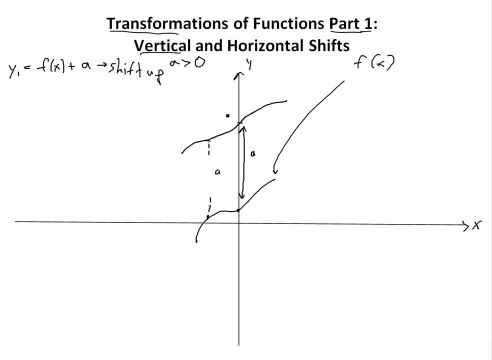 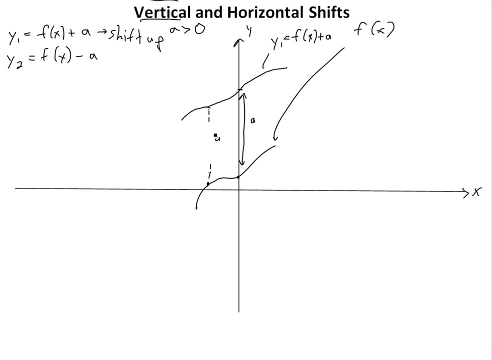 Up. So that's all it is. We're shifting up. And this, this would just be: y1 equals f of x plus a, x plus a. So let's look at well, another one, Let's y2, this one is f of x minus a. Now, this one is: this is exactly the same as this, except now, at every point you would minus a. 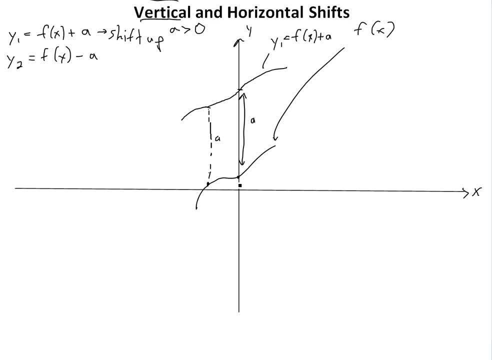 f of 0. is this, then it's f of 0.. So we're just going to go down down minus a. So this would be here. This would be minus a All the way here. So then this one, we're just going to shift all the way down again. 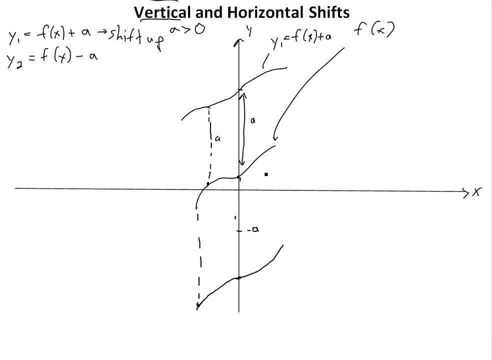 So basically it's the exact same, except we're shifting down, And this would just be: y2 equals f of x minus a. So we got this one, And this one is just shift down. This is pretty basic Shift down. So now we're going to look at: 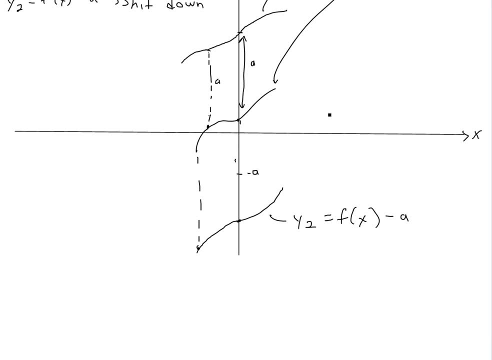 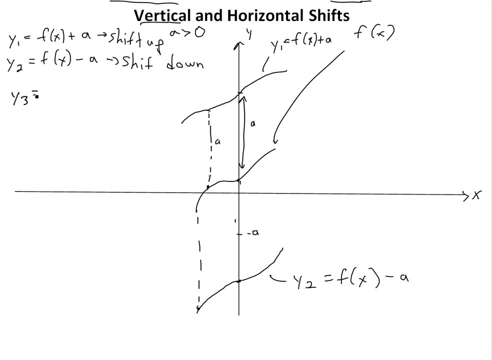 let's look at something else. Let's look at, let's say we had y3 or even- I'll just write it even up here. So let's say we have now equals f of x, x plus a. So now we're inside the brackets. So what this means is let's say if we have something like, let's write it down here. 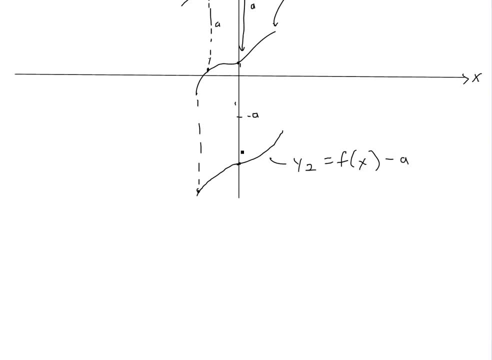 Let's say we have- I won't even shift it down here. Let's say we have f of 0. This is f of 0. So we, we know that's f of 0. So let's let's try to get f of 0 from yx3.. So so f of 0 in y equals 3 equation. 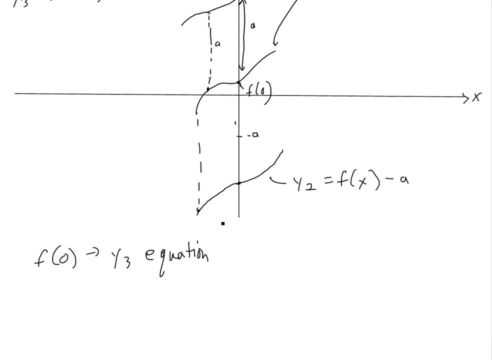 To get f of 0, we just have to make: well, basically x plus a equals to 0. And so then x equals to negative a. Let me just solve it. Yeah, so that that's what it means. So basically, at x equals negative a, we get. 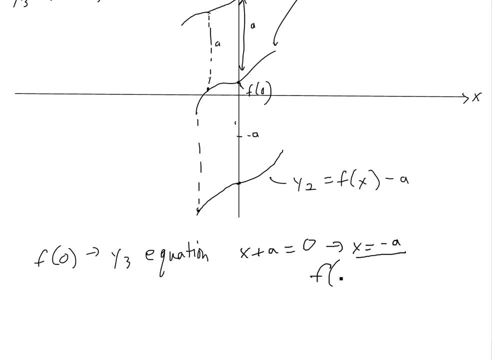 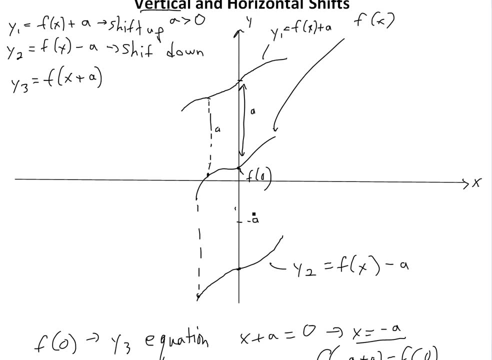 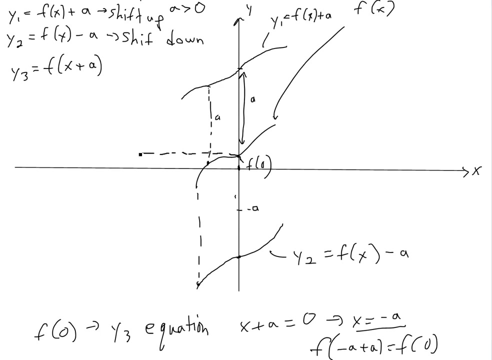 f of 0. So that's basically f of, yeah, negative a plus a equals f of 0. So basically, that's what x is equal to. So then, so here we're shifting negative a. So here's f, this is 0. So to get this one we're shifting. actually, yeah, we're shifting all the way here. 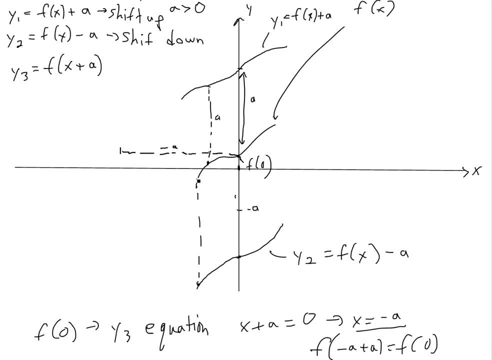 which is negative a. So we do that for every single part here, actually. So now all all this is is a shift to the left, And then this would just be: yeah, f of 3.. y3 is x plus a, So then this one is a shift left. 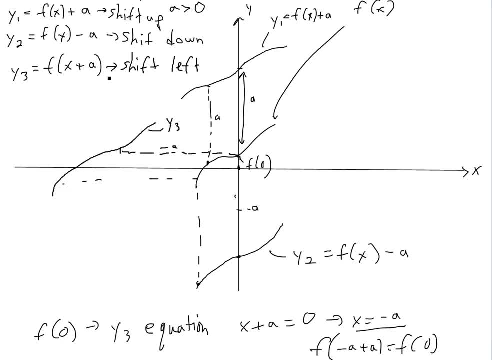 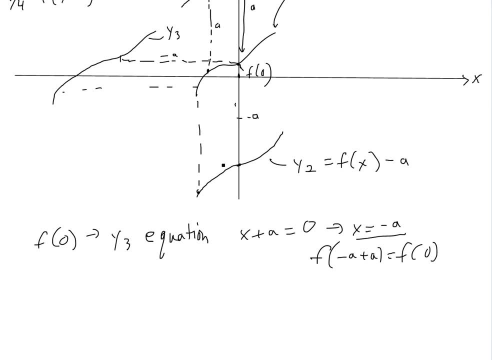 And then if we have, let's say, y4 equals f of x minus a. So this is similar to this one. We just make x minus a equals 0. And then x equals a. So then this means that at f of a, 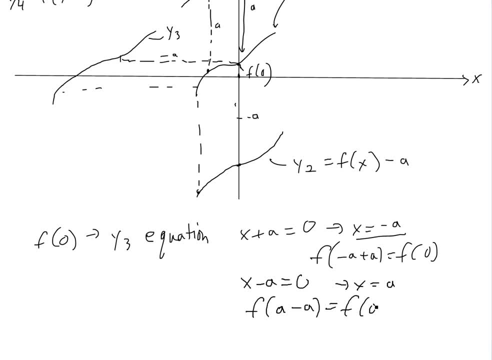 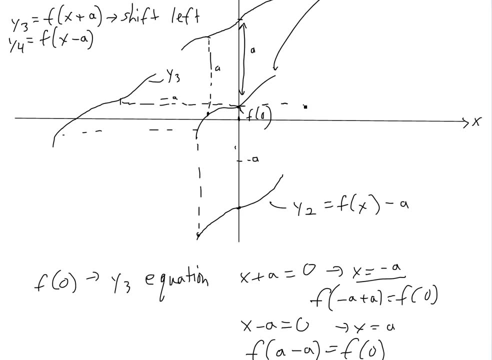 minus a, we get f of 0. So basically, at f of 0 is here, this is for f of x. But then to get that we need to shift a all the way here. So then we shift plus a. 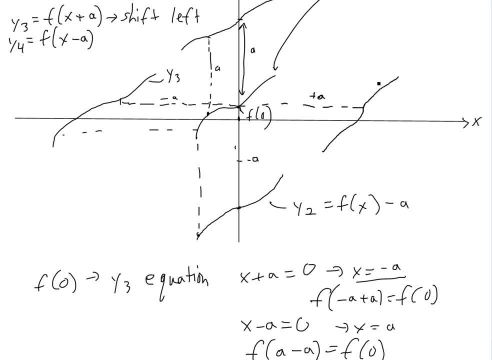 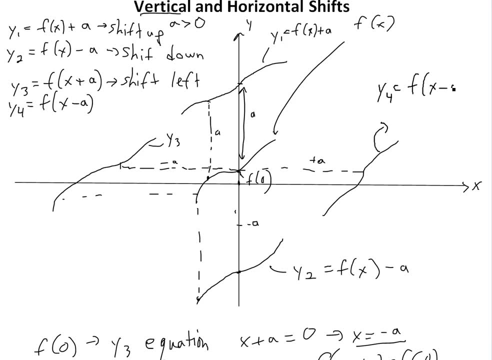 And then we get something like this: We do that for every single part of there, So then we get a shift to the right. This is: y4 equals f of x minus a, And then this one is shift right, Okay, so yeah, that's basically the shifting: vertical and horizontal shifts. 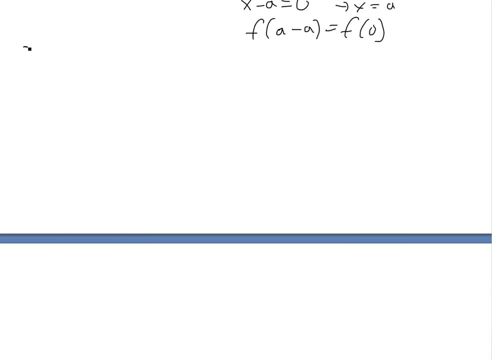 We'll do an example here. Let's look at, let's go, let's say: f of x is equal to x squared, So, and then this one is would look like this: So this one just looks like this. That's basically f of. yeah, this is just a parabola. 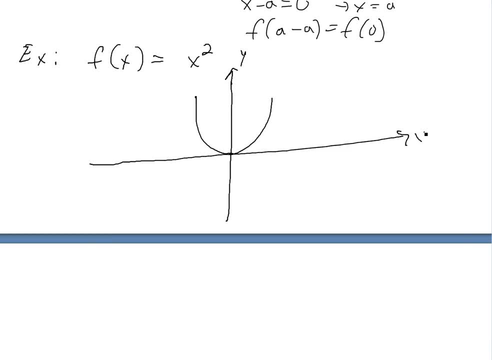 And this is y, This is x. It's a bit off, but yeah, then this is: yeah, this is x squared. Let's say we want to graph. yeah, basically, let's say we want to graph f of x. 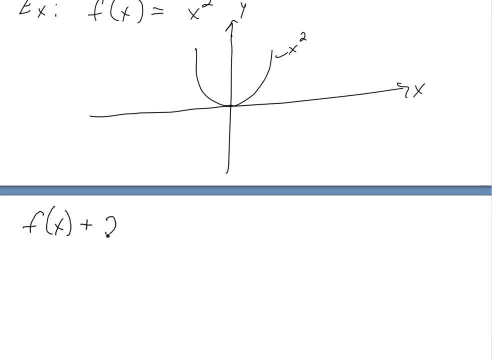 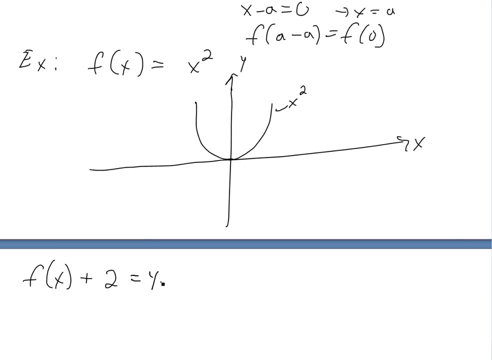 Let's say plus. let's say plus, yeah, plus 2.. So in this one, all we're doing here is just shifting. So let's say: this equals y2, or whatever. So again like before, this is f of x, f of 0 is 0, so we shift 2.. 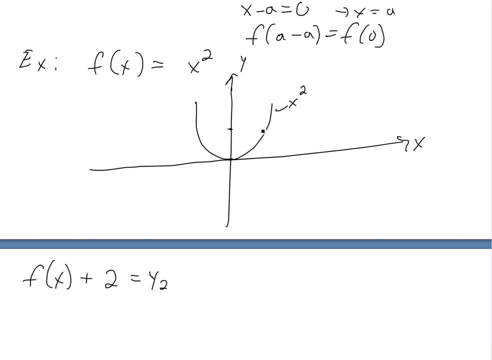 So f of 1, this is, let's say: yeah, 1 squared is 1.. So 1 squared equals 1.. So we go here, but then it goes to 3.. So this is 3.. So that's 3, and then it's basically going to be like this: 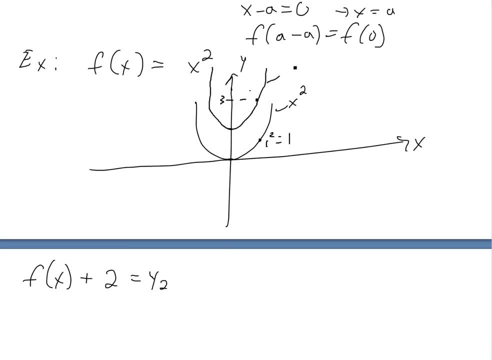 And similarly for this: yeah, this would be x squared plus 2.. Yeah, this equals to x squared plus 2.. And then this one would just be down here And then, yeah, And if we were to do a negative 1, it would just be shifting it downwards, like this. 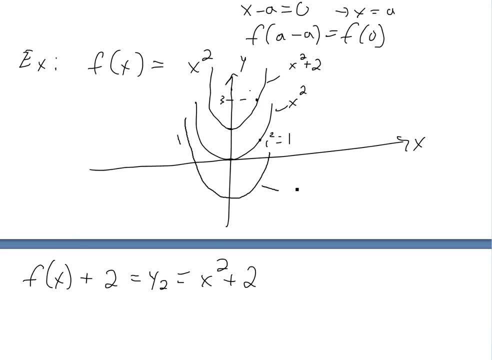 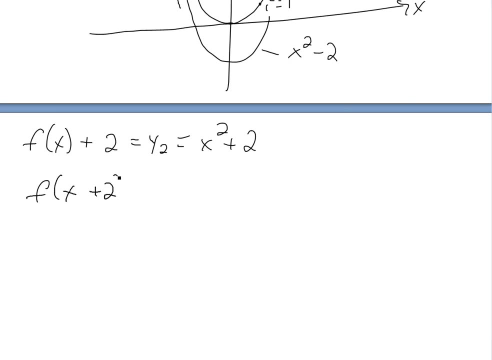 So it would be something like this, And this would just be x squared minus 2.. So let's say we want to graph, actually let's go f of x plus 2 inside. So then we just all we do is put it inside the f of x. 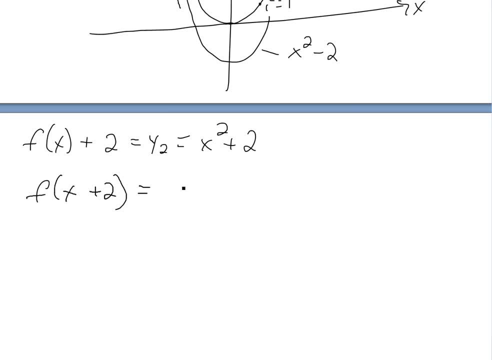 So we know f of x is x squared. So then we're going to get inside. the x becomes x plus 2.. So we'll have x plus 2 squared And, like before, this is just a shift. This is a shift left. 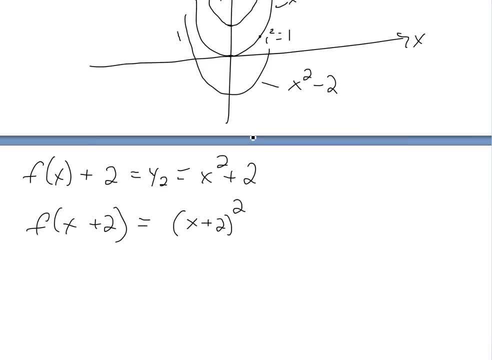 And then. so we'll just go 1, 2.. So we'll just draw it here. Draw this one- This will just be a rough outline of it, So that we have: this is x squared. This is y, This is x. 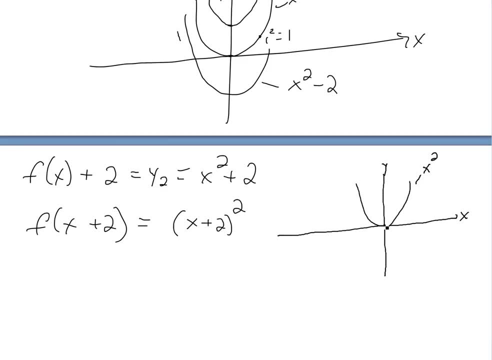 So basically, here, this one, we're just going to be going left 2.. So we go 0.. This is 0.. This is 1, 2.. So it's going to be something like this, And this is: yeah, x plus 2 squared. 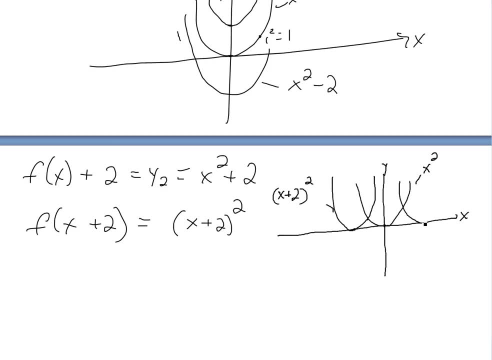 And similarly, if we go the other way, it's going to be like this: And this is x minus 2 squared. So just remember that negative is actually shifting to the right, Positive is actually shifting to the left Because you've got to make it equal to 0.. 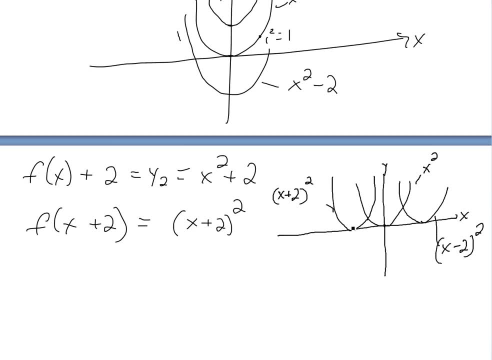 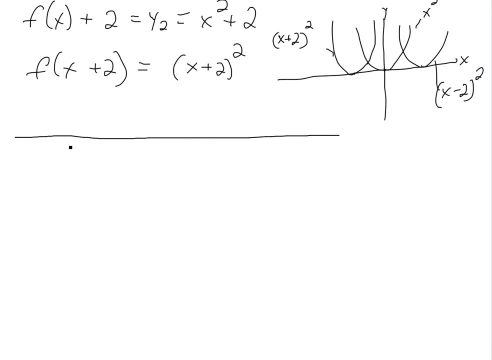 To make this equal to 0,, you put a negative 2.. And now this one, you put a positive 2.. So that's, and let's just get a let's go a hard example here. Let's go Graph, this one. let's say graph x3 squared plus 16.. 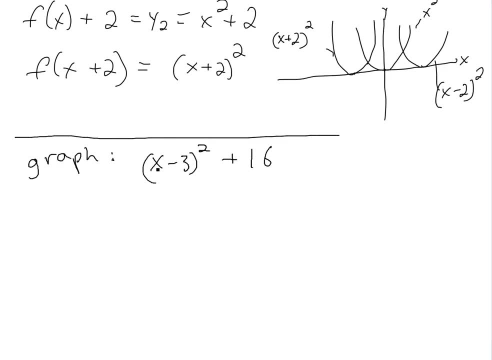 So now we know that, if you look at the basic one, we know that this is a transformation of x squared. This is a transformation of x squared. That's all we're doing is putting in: yeah, this one. all we're doing here. 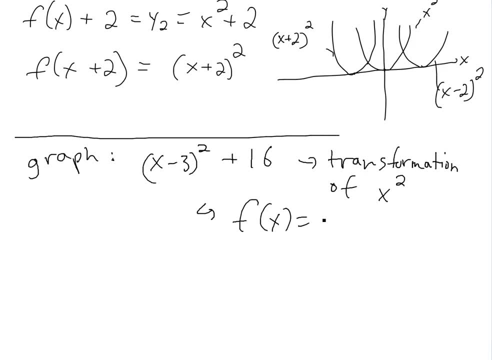 is just: actually, if f of x equals to x squared, then this function is just: we'll call this. let's say, yeah, this would just be f of x minus 3 plus 16.. So that's all we're doing is shifting this function. 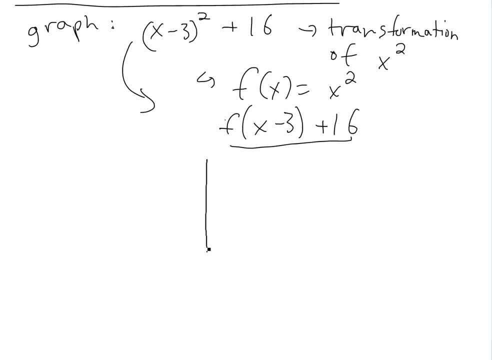 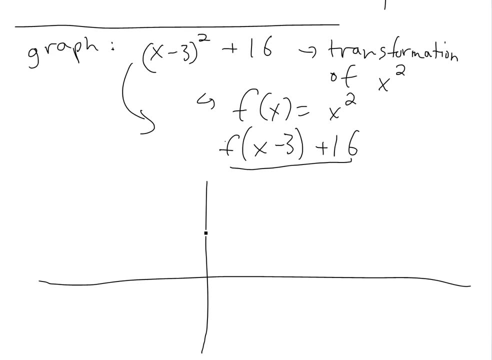 So if we for the graph, this one is very easy. It looks complicated but it's very easy. So you just go like this: So you shift 16 up, So we go shift all the way up and yeah, so this is. 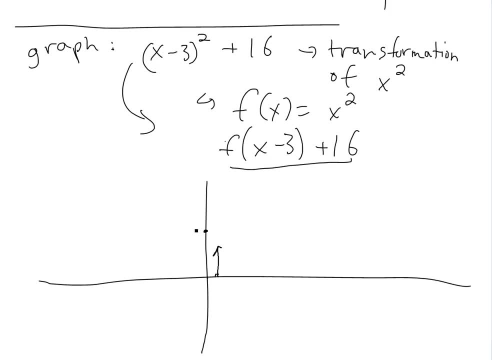 yeah, so we shift all the way up. this is say: this is 16.. This is y and this is x. and then we: this is negative. so we go to the right, We shift right 3.. So we shift, let's call this 3.. 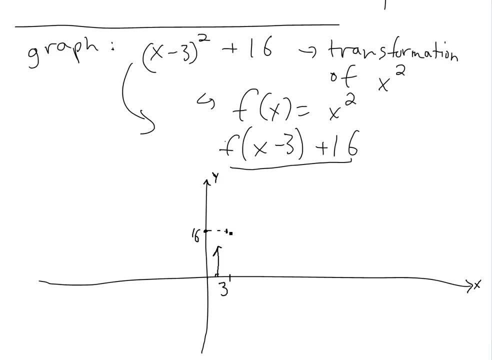 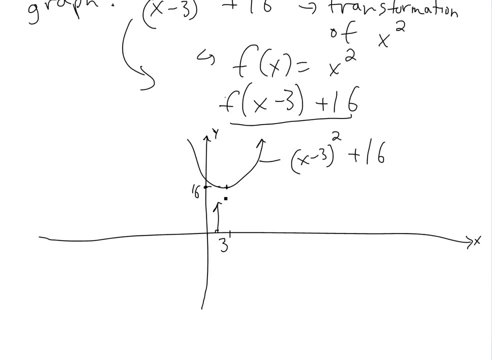 So we go up and then we go right, and then it's going to be a problem. So there you go. This is very easy, And this is just: yeah, x minus 3, squared plus 16.. So basically, yeah, whenever you're graphing something, 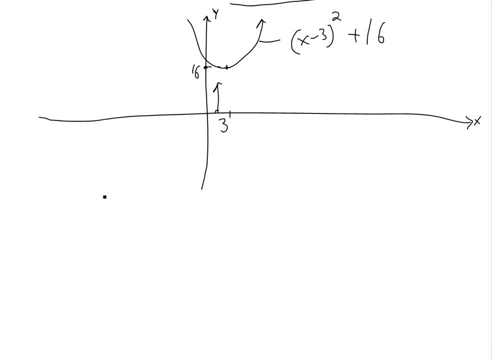 just quickly in your mind, remember to just as a hint: yeah, it might be. yeah, just look at the basic function. Look for, let's say, yeah, basic, yeah, basic function inside the complicated one. So in this example it's just x squared because it's probably yeah and there's an x squared. 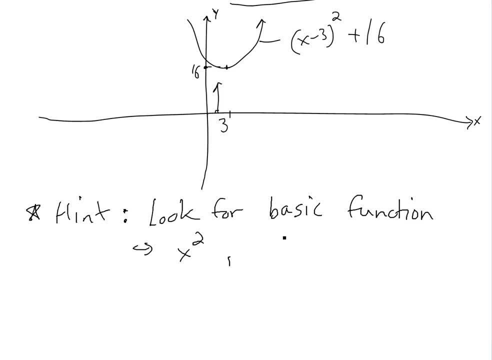 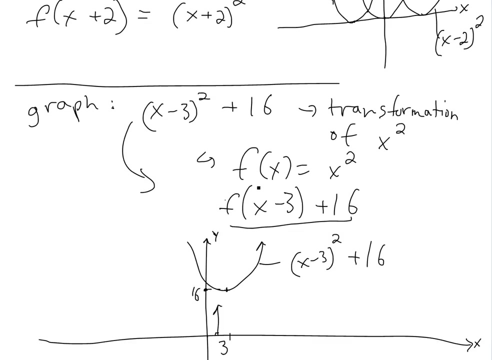 and it was just a transformation of it. And then, yeah, that other stuff was just a transformation, Just a transformation, Yeah. so basically, if you understand this transformation of all the functions, you can graph like many other ways, and then all you got to know is just the basic one. and then 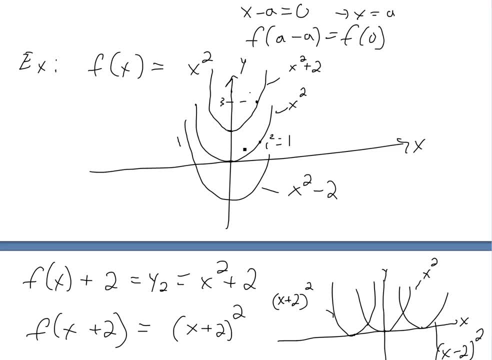 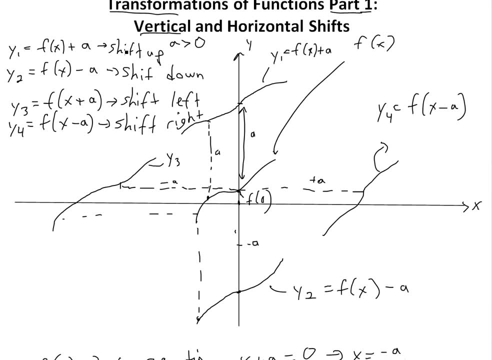 just how to shift it, how to whatnot. I'll show you straight. I'll show you the stretching of them later in my part two series. Well, thanks for watching. Hopefully you learned. and this is basically, if it's plus a shift up, minus a shift down. 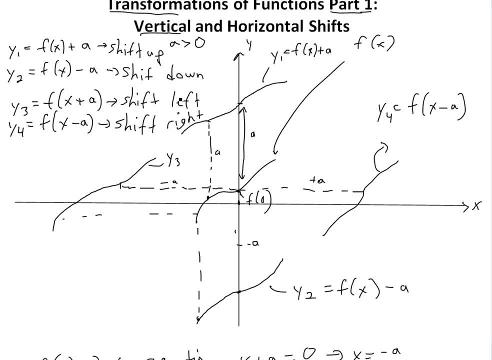 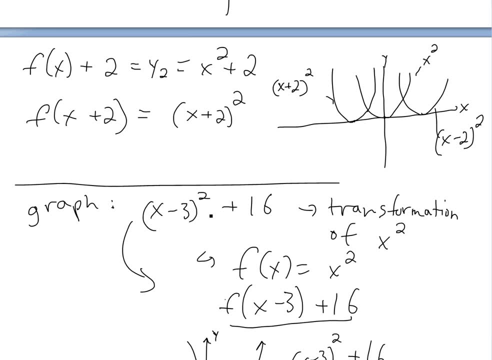 If it's inside, plus and minus are actually opposite. Plus is left, minus is right. So that's all it is, And then you could use that basically to find out what your basic function is in this case. In this case, it's just x squared. 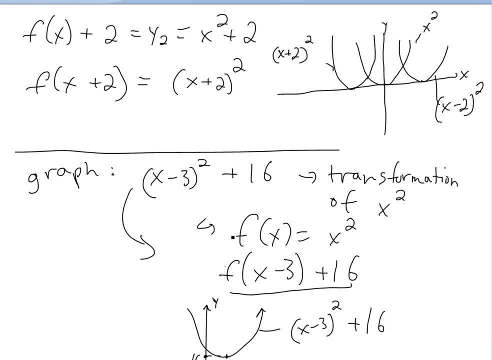 These are all just transformations of it, and then you could graph it easily. Well, thanks for watching and stay tuned for another math easy solution. 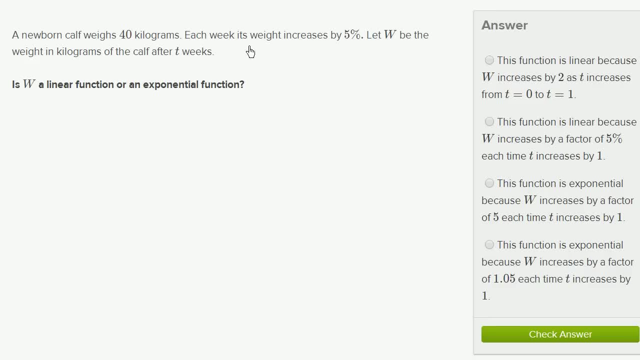 A newborn calf weighs 40 kilograms. Each week its weight increases by 5%. Let w be the weight in kilograms of the calf after t weeks. Is w a linear function or an exponential function? So if w were a linear function, that 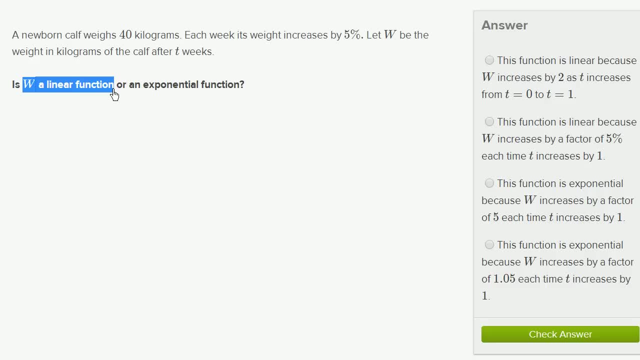 means that every week that goes by the weight would increase by the same amount. So let's say that every week that went by the weight increases. Or really they're talking about mass here. Mass increased by 5 kilograms. Then we'd be dealing with a linear function. 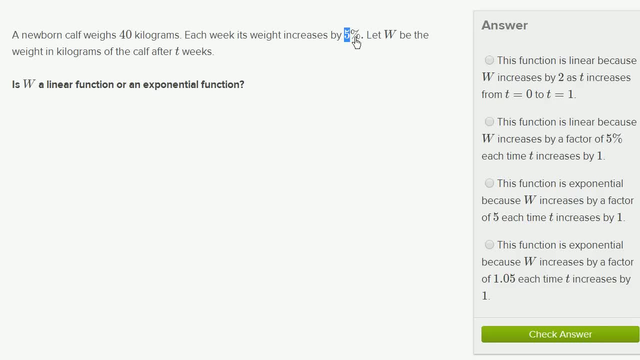 But they're not saying that the weight increases by 5 kilograms. They're saying by 5%. So after one week it'll be 1.05 times 40 kilograms. After another week it'll be 1.05 times that. 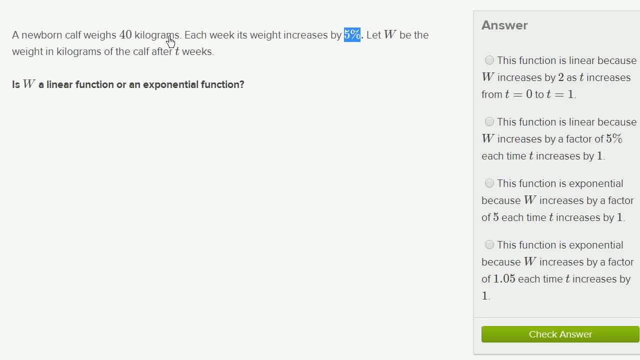 It'll be 5% more After the next week. it'll be 1.05 times that. So really, if we really think about this function, it's going to be 40 kilograms times 1.05 to the t power. 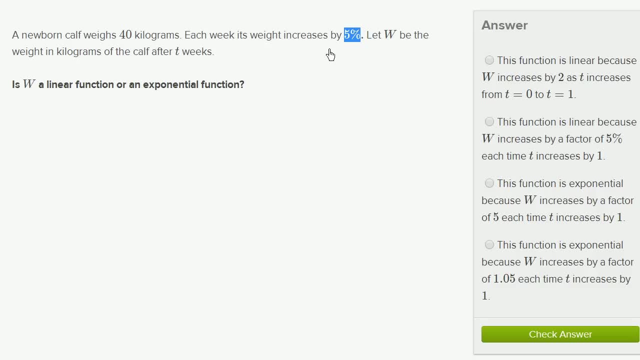 We're compounding by 5% Every time. we're increasing by a factor of 1.05.. Another way of thinking about it: by a factor of 105% every week. So because we have that growth by a factor, not just by a constant number, that 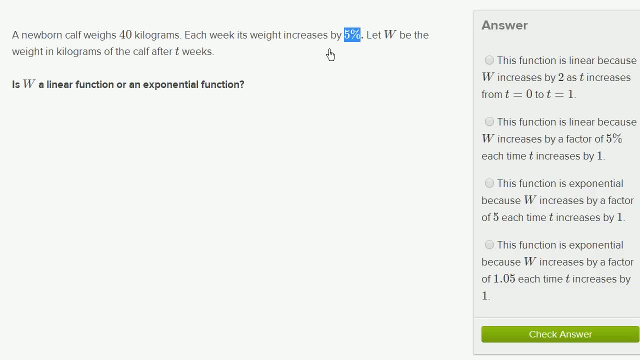 tells us that this is going to be an exponential function. So let's see which of these choices describe that This function is linear. No, we don't have to even read that This function is linear. Nope, This function is exponential because w